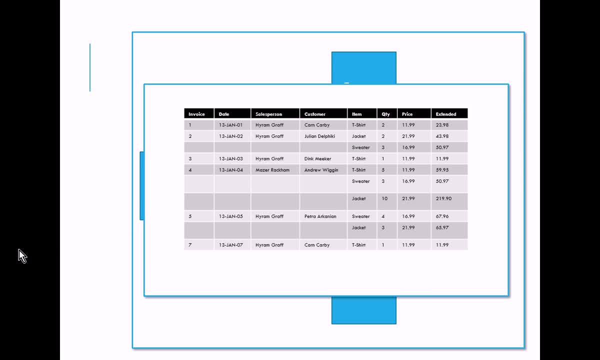 this might be a system for ordering goods online, or it could be an invoicing system or just products, And I use this example because most of us are familiar with ordering things and how invoices work and so forth, So this might be an artifact that we saw. You can see here. 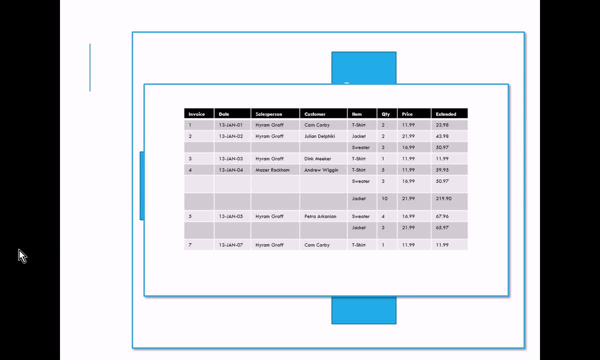 it's a list of invoices. One thing you'll notice if you take a look at invoice number two: it has more than one item on it. That's why there's a blank line there. So this is just some raw information that somebody gave us as a form, And when we look at that we can break this. 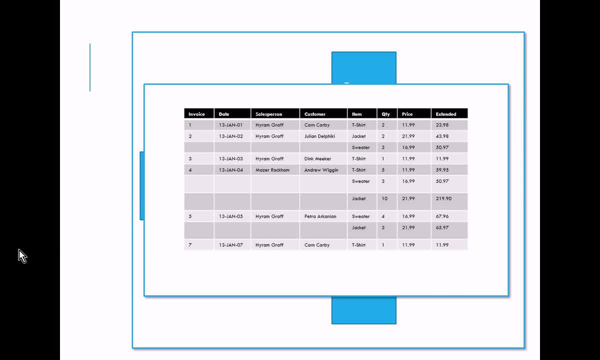 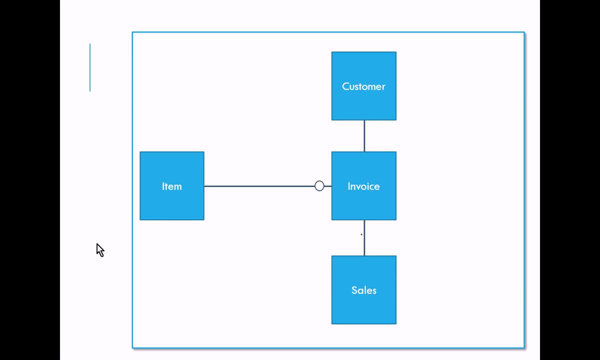 into or we can, along with all of our other analysis, we can basically put this together to try to come up with With a database design. So, for example, we would have looked at that artifact and we would have figured out that one of the main topics is a customer, Another one is the invoice, Another 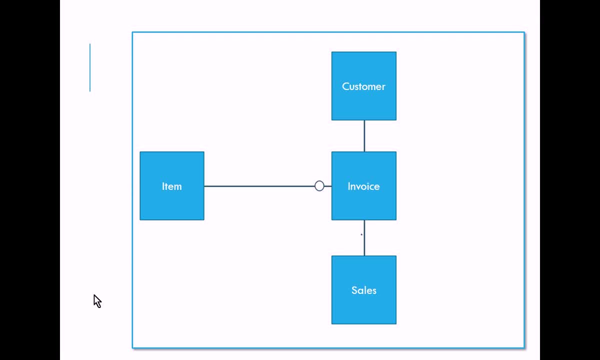 one might be salespeople And another one might be the item itself which appears on the invoice, And we would start to diagram this and figure out what the relationships are. So we might say that the customer and the invoices relationship, So the invoice has one and only one customer And 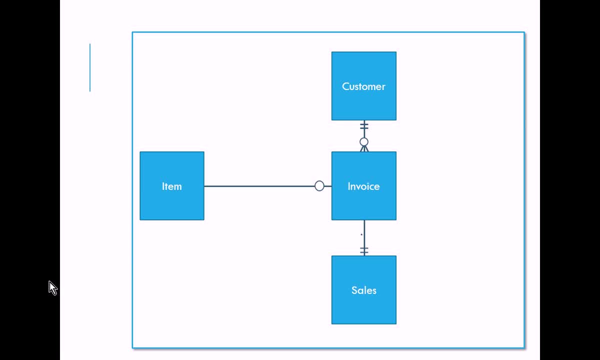 we would have zero or many invoices. An invoice can have one and only one salesperson, but a salesperson could have zero or many invoices- hopefully more than zero, or they won't be a salesperson for very long. And then our invoice has one or many items on it And our item can be. 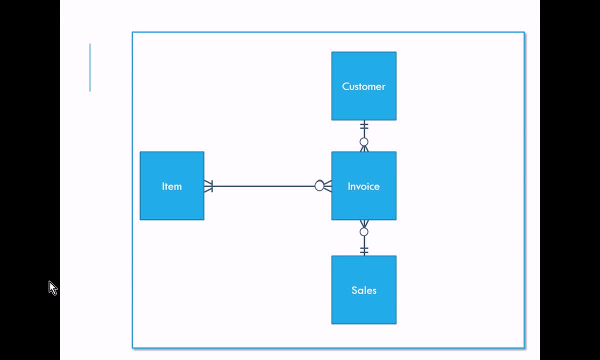 on zero or many invoices. There is one problem here. When I talked last time when we looked at logical design, one thing I did mention is that in a physical design- it would be a physical design- It would be nearly impossible to have a database with a many-to-many relationship. And here we have. 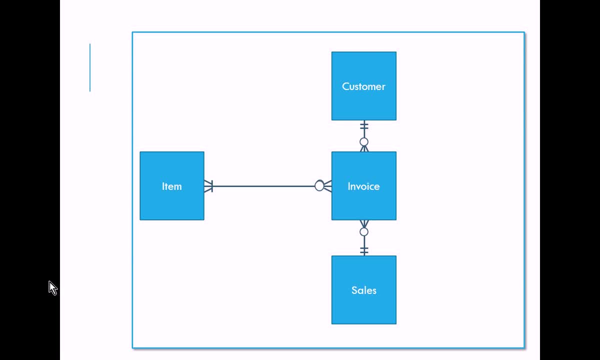 a many-to-many relationship between the item and the invoice. So what that typically means is we need to create a new entity between those two to handle that many-to-many relationship, And I want to show you how to add those. It's very simple, So anytime in your diagram when we start moving. 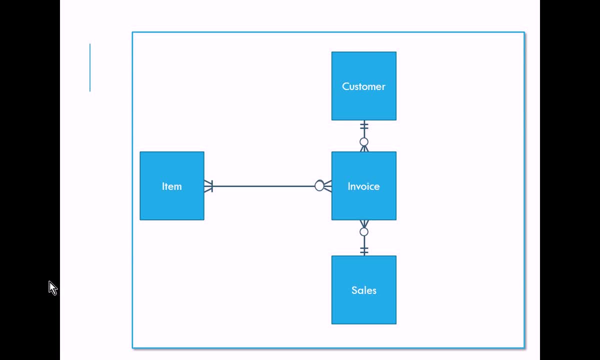 into the physical design and before we even start to normalize, the first thing we're going to do is look at that logical design that we did before and say, okay, where are all my many-to-many relationships? And you're going to start to put in those many-to-many. 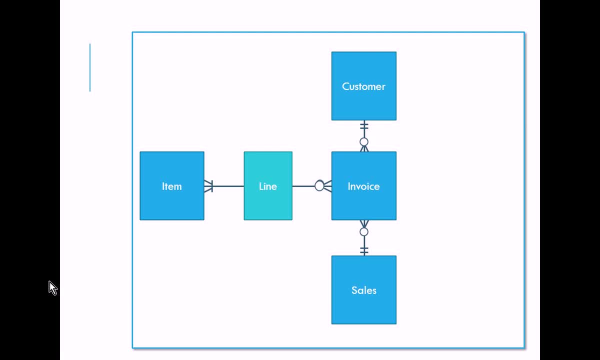 relationships, some kind of a linking table. So in this case I have line for my linking table. This might be the line items on an invoice. Think about when you go to the store and you get a receipt. you have one receipt but that receipt contains many items on it. has line items on the. 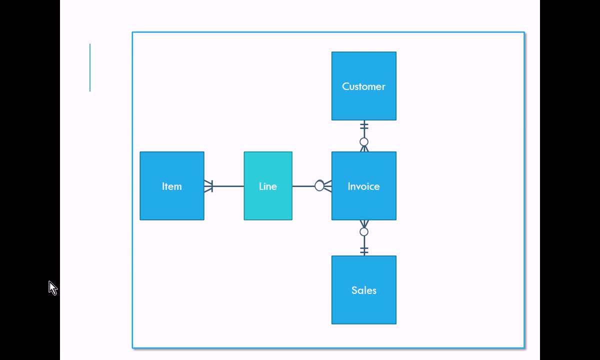 receipt which have something like a quantity and the price of what you're paying on that receipt in addition to the full price which would appear perhaps in the invoice. So when you insert that helper table or that linking table between the other two at the many-to-many, 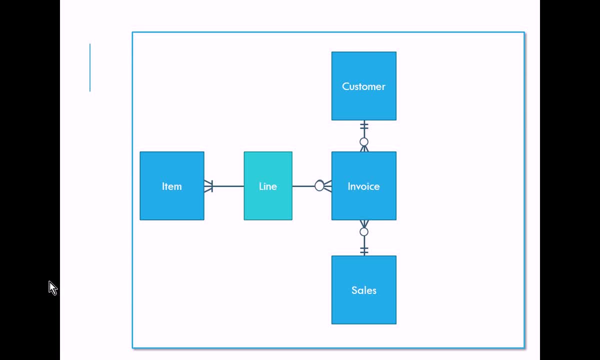 relationship. the next step is: how do I now convert this to one-to-many relationships? The first thing you do is take your relationships and you pull them across. So let me show you what I mean. So I'm going to pull the relationship from the item across the linking table and I'm going 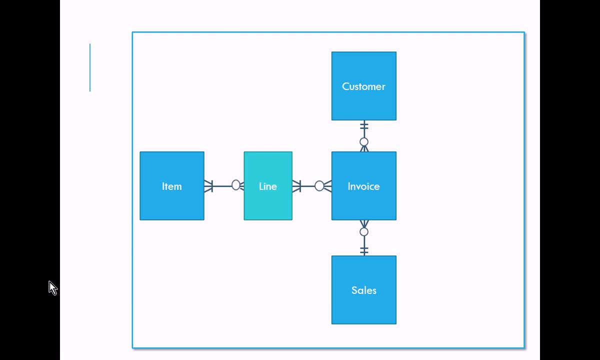 to pull the one on invoice across to the other side, like so. So I kind of just used those two relationships and I pulled them across and I'm going to pull the one on invoice across to the linking table. Then I replace the other ones with a one-to-one. So the two relationships. 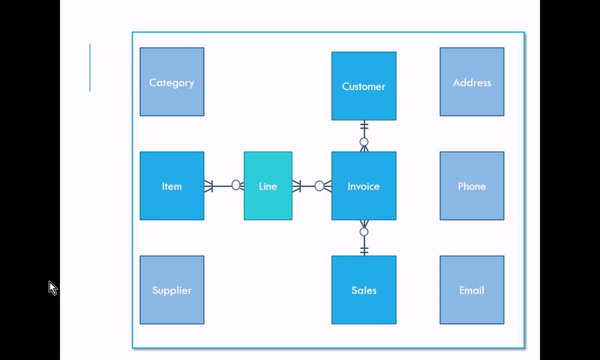 and it may not be in my diagram here, but those two relationships on the ends against item and against invoice would turn into one-to-ones. So an item can have zero or many lines, and a line would have one and exactly one item. Likewise, a line would appear on one. 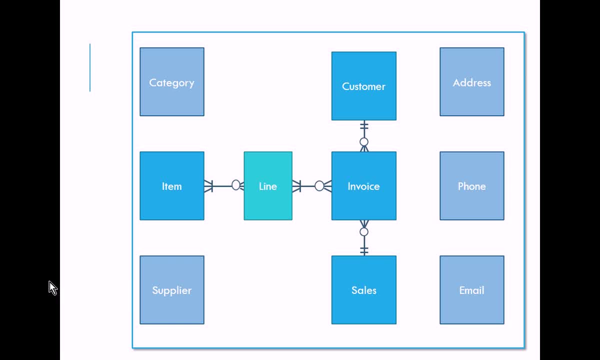 invoice. It can never appear on more than one invoice And an invoice can have one or many items. So that's basically what it looked like And of course, we would have other relationships to worry about. Customers might have addresses and phone numbers and emails. Items might have 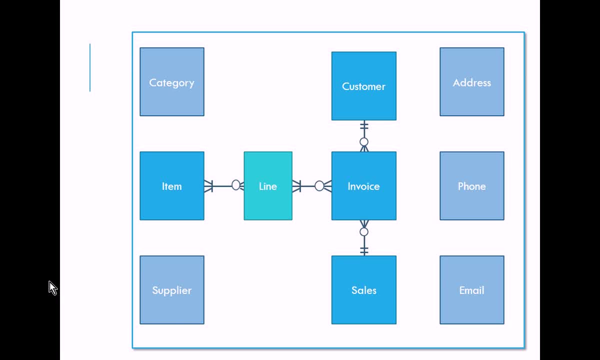 suppliers and categories and things like that. So other items might come out of the woodwork here as we move forward with our design. I just wanted to show you that technique for how to connect those together And then I kind of wanted to show you when you get to a physical design- this diagram: 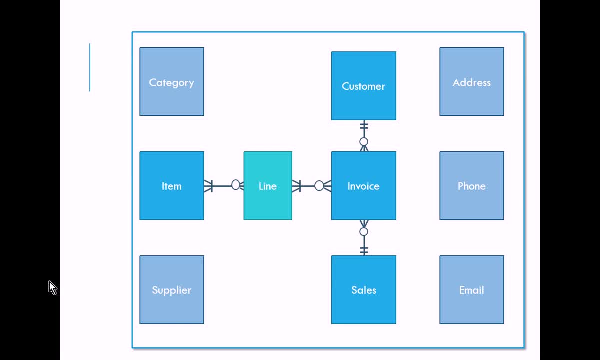 that you see here with the item, the line, the invoice, the sales, the customer. this is what it's going to end up with. So I'm going to pull the one on invoice across to the other side, looking like in our database. So you've got in the middle here, right in the middle, that table. 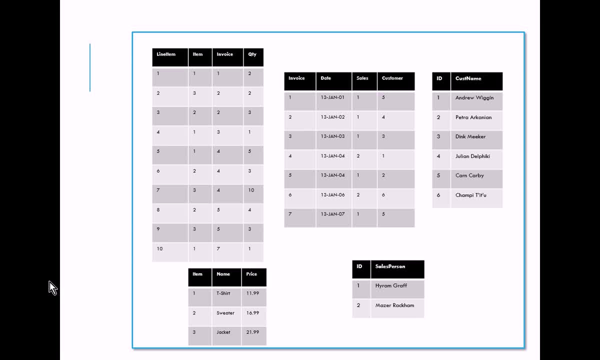 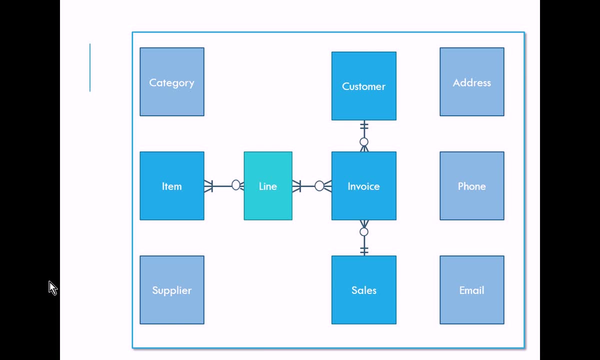 that has the invoice number on it. That would be our invoice table, which is kind of connecting everything else. If you look over here, my invoice table is sort of in the middle and everything else sort of connects to that, So that one's in the middle. Notice that each one of these tables 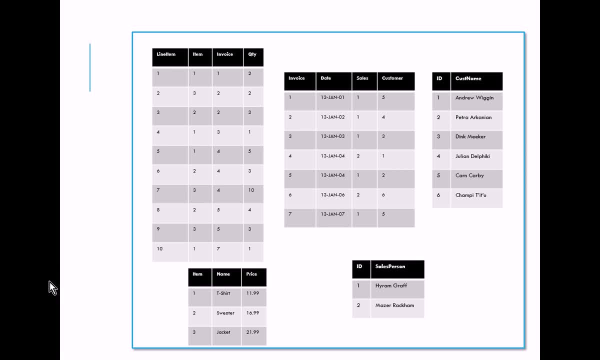 also has a primary key. For instance, in the invoice table it's the invoice number, For the salesperson has an ID, a customer has an ID. The first column in each one of these tables is the primary key, But in addition there is a foreign key. So if you take a look at the line item, 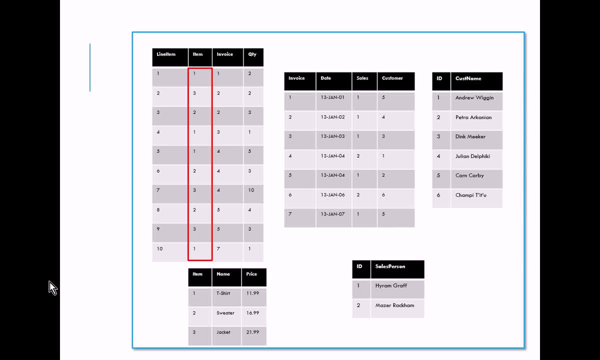 there is a foreign key in the line item, So it has the item number for each line, So every line has an item And that references to the item table, to the primary key in the item table. Likewise, there's an invoice number for each line which tells us which invoice that line item. 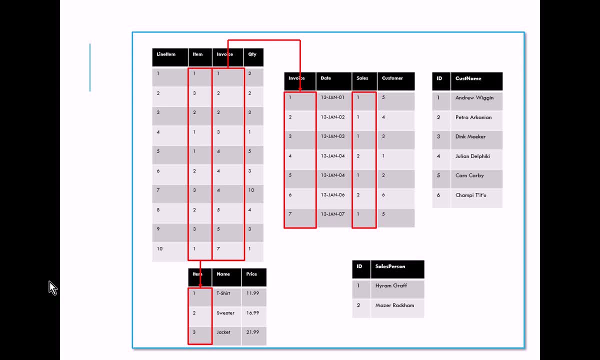 belongs on And likewise our salespeople here on each invoice and it tells us which salesperson it is. And our customer ID is on the invoice and that tells us which customer we're looking at in the line item. By combining 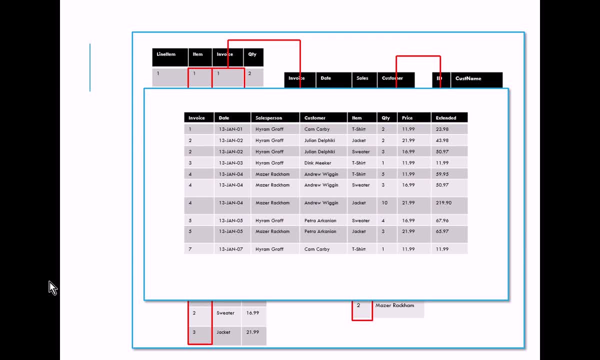 all these tables, I basically get back what I started with. So here is the kind of that artifact I showed you in the beginning. We can basically get back to that. eventually, After we do all this design, we end up getting back to what the customer really wants. It's something similar. 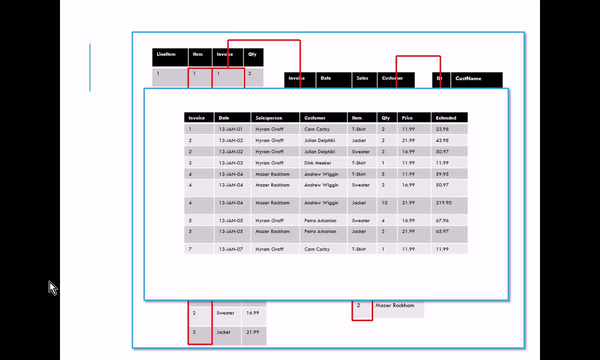 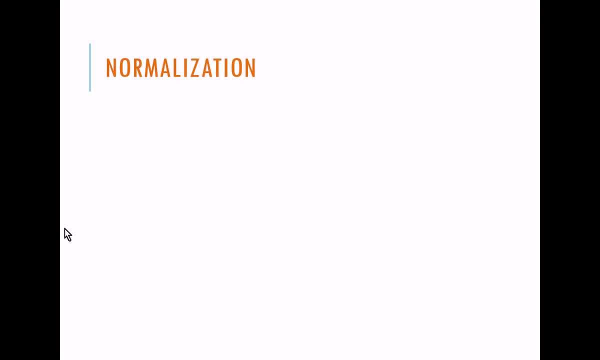 to that artifact we looked at before, but now we have a way to store all this stuff in our database. So now that we have a general idea of how all this works, let's talk about normalization. So once we have that logical design and we've got all those relationships, we've fixed our 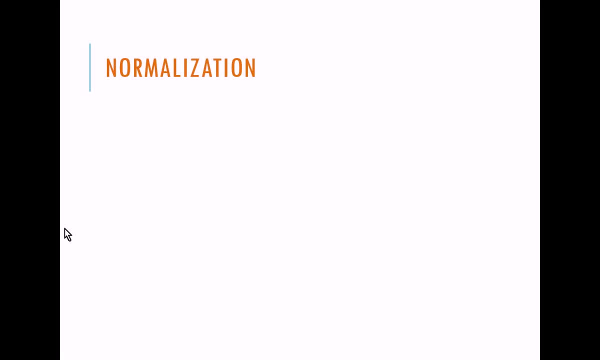 many-to-many relationships. we started thinking about our foreign keys and I'll talk more about the foreign keys in the next video, how we're going to place those foreign keys. But you don't have to worry about that too much yet. We do have to start doing normalization. What exactly is? 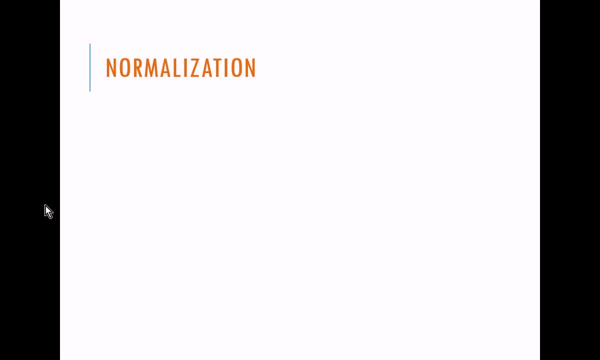 normalization. So normalization is the process of removing potential anomalies from the database design. So these anomalies include: there are three anomalies we talk about in most database courses. We talk about insertion anomalies, update anomalies and deletion anomalies. What is an anomaly? An anomaly is some kind of an error. 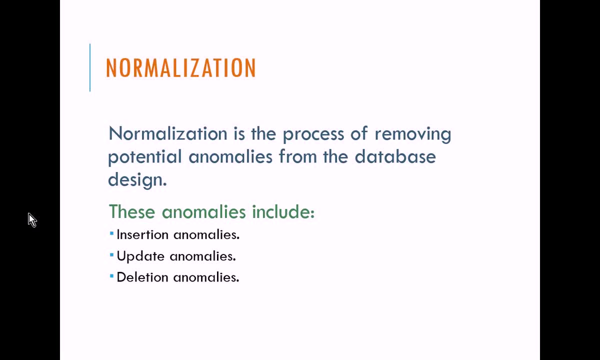 or something that can happen that can cause corruption with our data or make it difficult to use the database. We want to reduce these anomalies or the likelihood that these anomalies are going to occur, So let's talk about each one of these. An insertion anomaly is an anomaly that 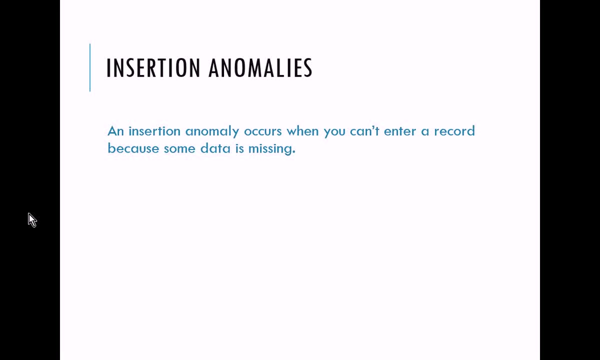 occurs when you cannot enter the database, or when you cannot enter the database or when you cannot a record because something is missing. So consider that we have a database and there might be a rule, maybe a business rule, that every employee has to be assigned to a project, Maybe it's a consulting. 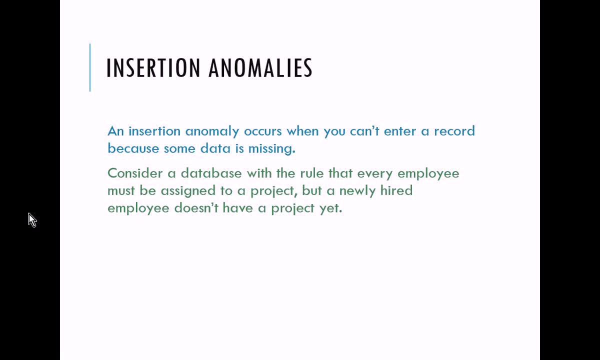 firm. If you're not working on a project, then you're not making any money for the company. So maybe that's a rule: You have to have at least one project. But your first day on the job, when you're newly hired, you're not going to have a project yet. So if you codified that business, 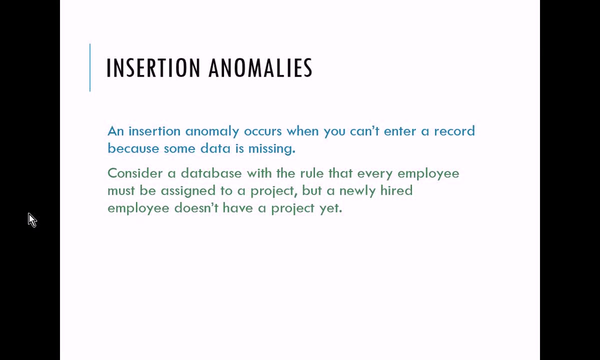 rule into your database and you say, okay, every employee must have a project. you're not going to have anything. you can enter into that table, yet You're not going to be able to add your new employee because you're not going to have a project to put them in. So that would be an 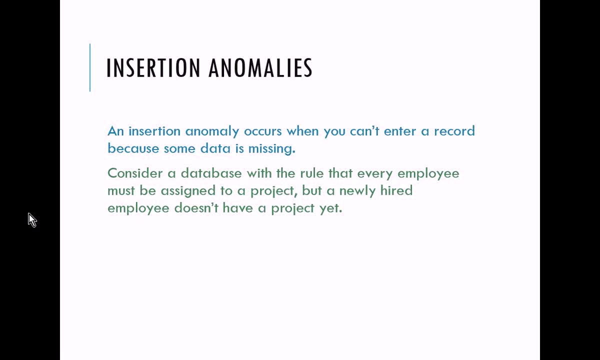 insertion anomaly. If we're prevented from inserting data because of the structure of the database, then that's going to be an insertion anomaly. So one solution: you could, somebody might. if we were in class, somebody would say: hey, Brian, why couldn't we just have a dummy? 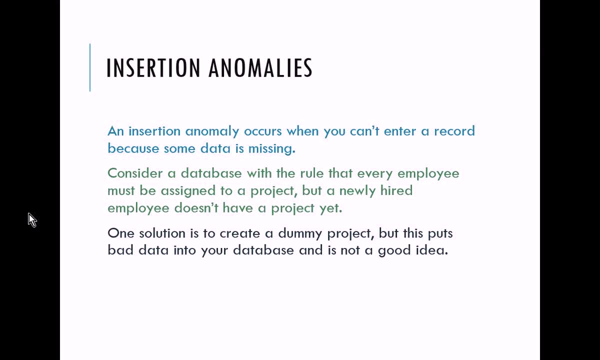 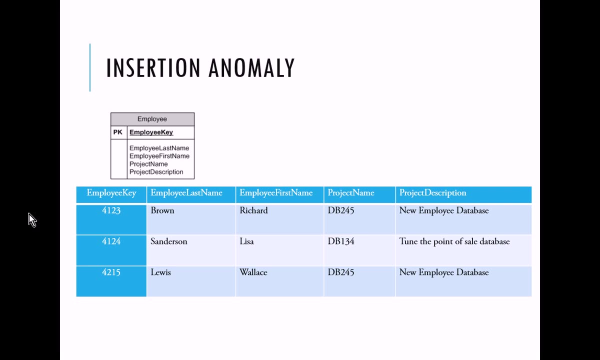 project. Well, because that's not really the best practice. We're essentially, from the very beginning, we're going to be putting bad data in our database, We're going to be doing kludgy workarounds right from the very beginning. So we don't really want to do that, And here's an example of that table. 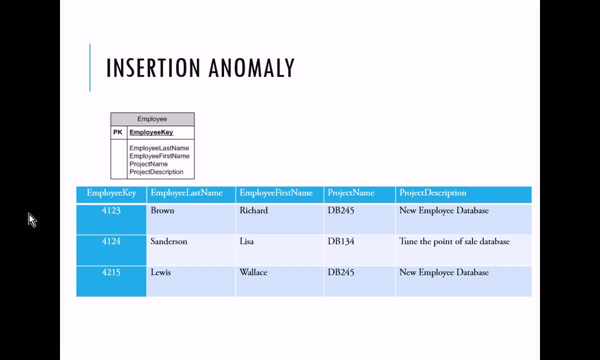 So here we have a project name in the database, So we have to put a project name in there. And if there isn't the project name, then we have a problem. There's nothing to put in there and we won't be allowed to insert data, So we're going to have to put a project name in there. 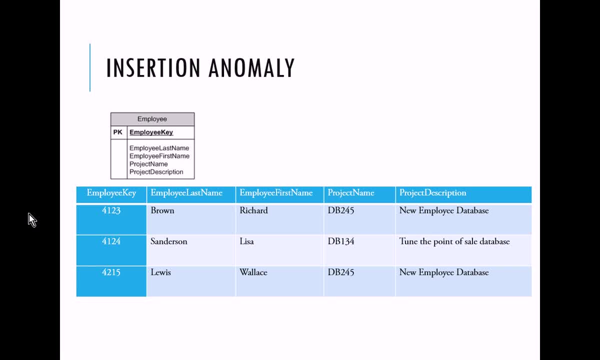 So that's certainly one example of an insertion anomaly And there are others. Usually when you have a one-to-one relationship that can cause an insertion anomaly and you have to be careful about those. So another type of anomaly is an update anomaly. Before I move to the next slide, 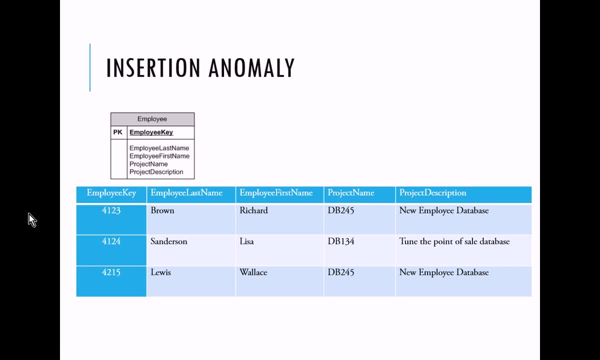 just take a look at this table and look at the project name. So the employee with the last name Brown- the first one on the list, their project is DB245.. And the employee with the last name Lewis is on project name Brown. So the employee with the last name Brown is on project name Brown And the 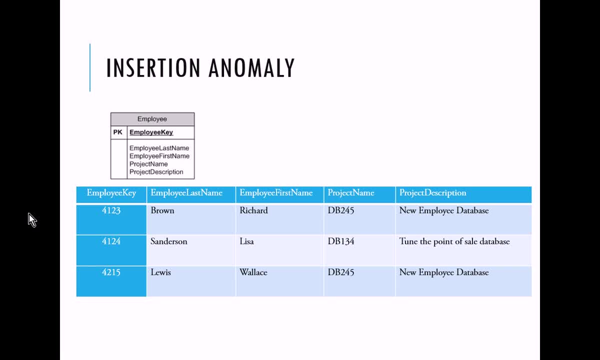 employee with the last name, Lewis, is on project DB245. But what if somebody decided to change the name of project number DB245? What would I have to do in this table? Well, the answer is I would have to go through and make sure that all the projects called DB245 are updated to the new. 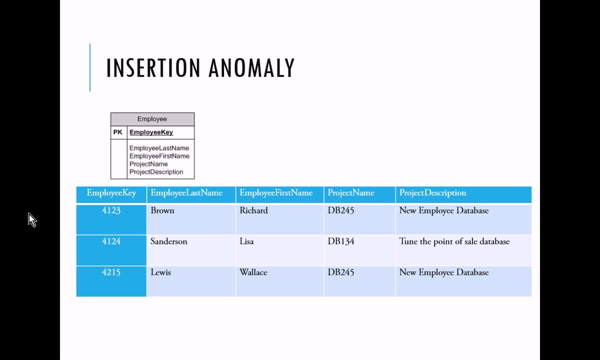 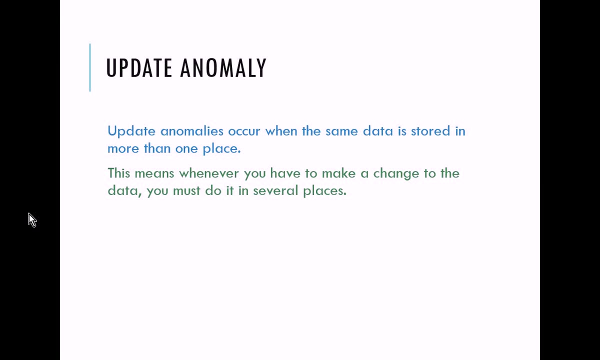 name. Maybe we're going to call it DB246 now or something, Who knows? For some reason we had to change it. That is an update anomaly. It occurs when the same data is stored in more than one place, And whenever you make a change to the data, you have to do it in several places. 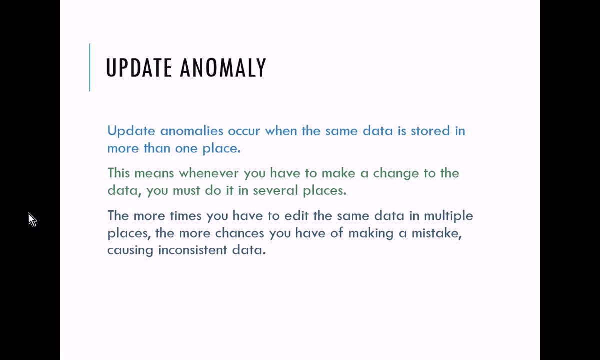 So that can cause errors over time, That can cause consistency problems. You know, over time you're going to get this drift from the source of truth for that data And things are going to start to get a little messed up in your database. So we don't want to do that. We don't want to have 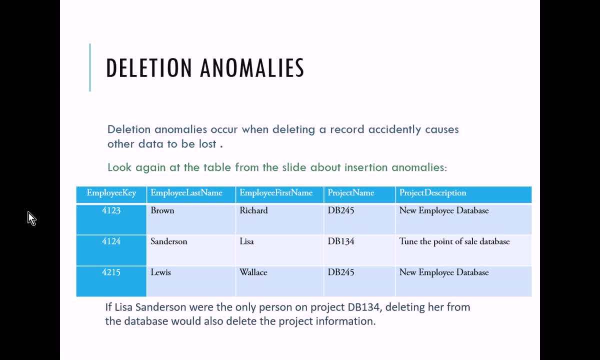 update anomalies. Another anomaly is deletion anomalies. This occurs when deleting a record accidentally causes other data to be lost. Going back to this example, Lisa Sanderson is my only employee in project named DB245. And she's the only employee in my project named DB245.. And she's 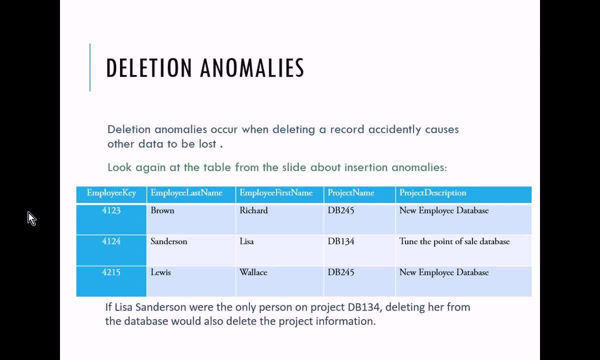 the only employee in my project named DB134.. If I were to remove Lisa Sanderson, so let's say Lisa Sanderson is leaving the company and I remove her from my employee database- there now is no trace of project number DB134.. It's gone, unless I have it in another table. So in this unnormalized 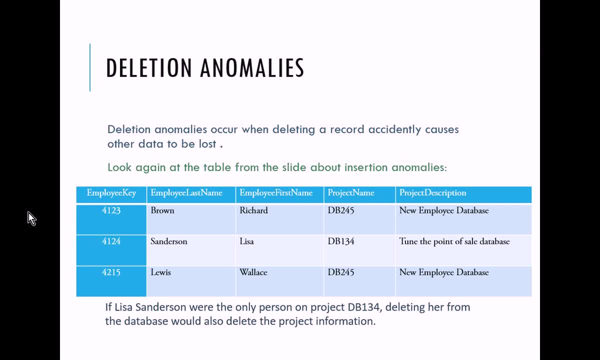 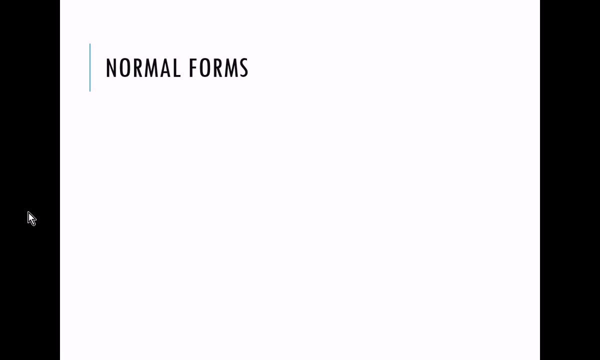 database that doesn't have a reference to that somewhere else. by removing that record, I've removed all traces of that project name, So now it appears as though that project doesn't even exist. So that's certainly a problem. We want to prevent that from happening. So, in order to get to the goal of not having all these anomalies and 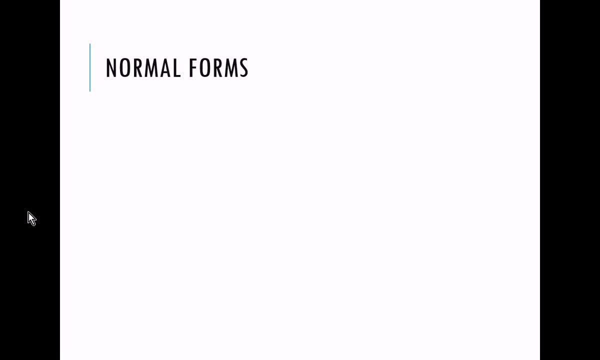 to help us do that, we have some standard methods of normalizing our database. There are these normal forms that have been created to help us address these issues, And I'm going to show you a list of those. We're only going to talk about the first three normal forms in this list, And those are: 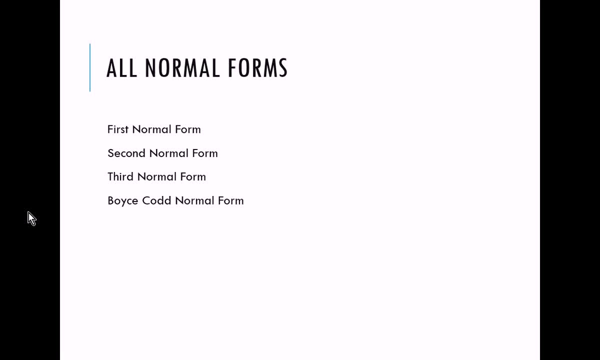 the first normal form, second normal form and third normal form. There are some additional normal forms like the Boyce-Codd normal form, fourth normal form, fifth normal form, domain key normal form and so forth, But we are going to stop at third normal form And I would say probably 99%. 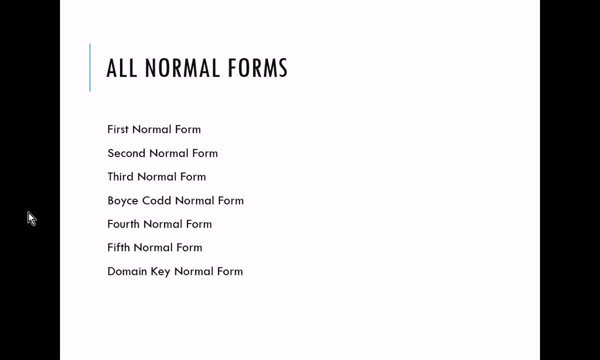 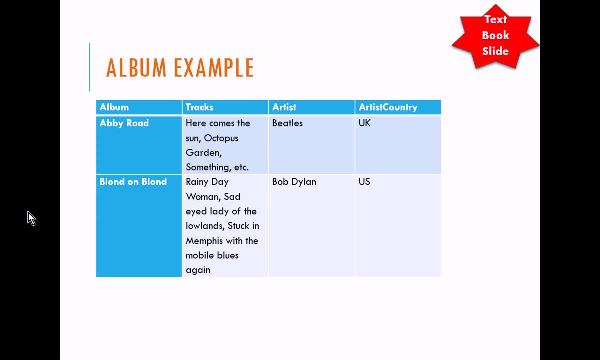 of the databases that I've designed in industry have usually gone no further than third normal form. In fact, sometimes we denormalize a little bit, which I'm going to talk to you about in this presentation. So some of these slides are from a textbook. These are from a Pearson textbook. 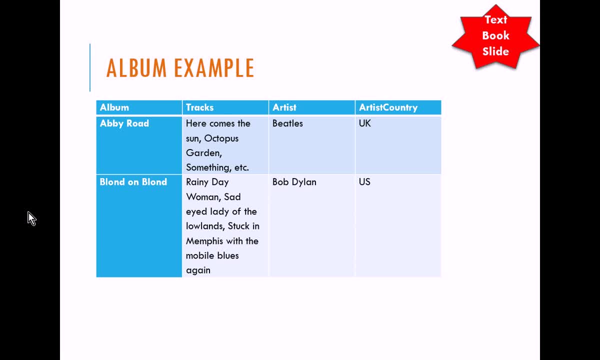 used in a course And this uses an example of a textbook that I've used in a course And this is an example of a database that is a music album. So in this particular case, we have an album called Abbey Road, another album called Blonde on Blonde, And each of them have many tracks, an artist and 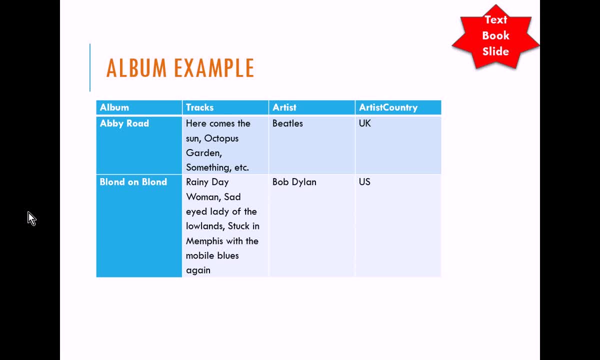 a country for the artist. This is an unnormalized table, So we start with this one table. It's not normalized, So now we're going to normalize this table. What do we need to do to normalize it? Well, the first thing is, if you take a look at the tracks column- 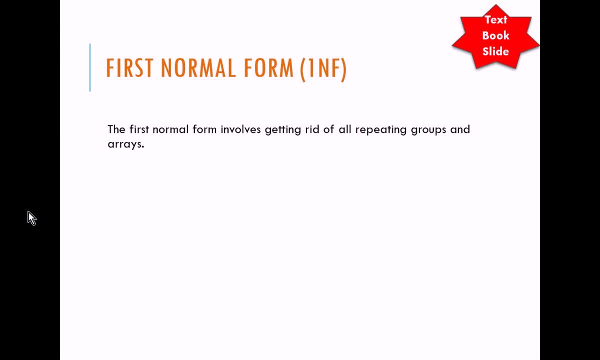 we have lots of tracks all stuffed into one column. So in order to achieve first normal form, we have to get rid of any repeating groups and arrays. So repeating groups are lists of things in the table, such as if you had more than one phone number, like a phone one and a phone two. 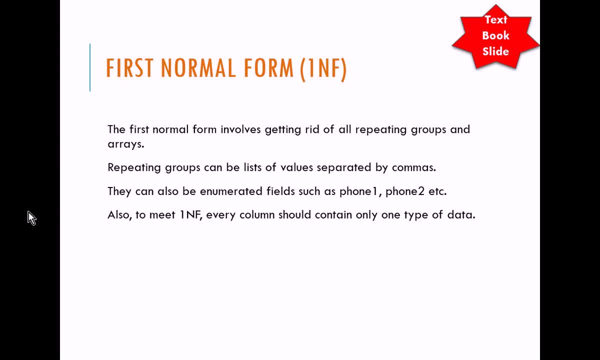 that's a repeating list in our table for each record, So you're going to look within each record. So if you look at a single record and there is a repeating value for a single thing, like our tracks on a record, then we are. 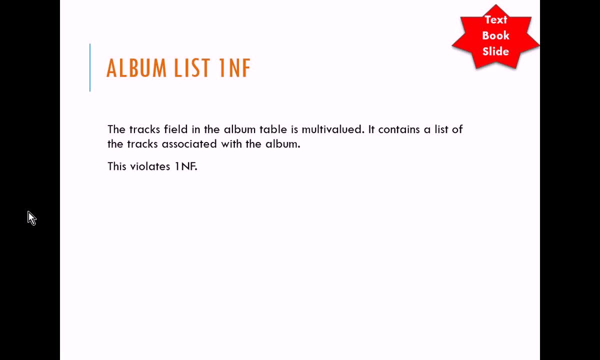 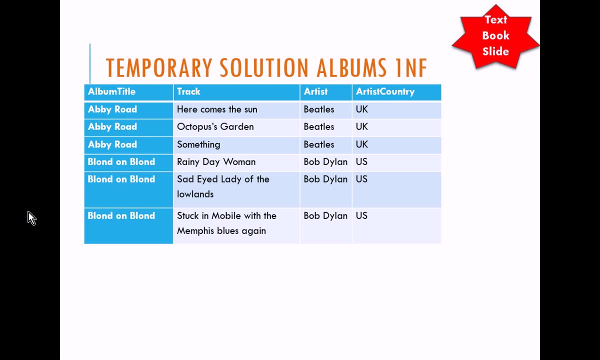 not in first normal form. We have to get rid of that. So in order to get rid of that, we're going to have to move our tracks to a new table, So let me show you what that looks like. So here we have a new table for our tracks, So we put the name of the track and the album title. 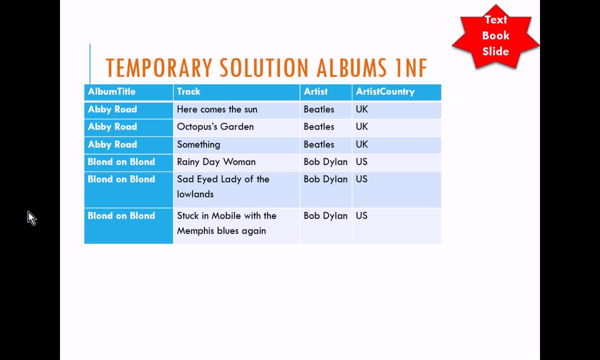 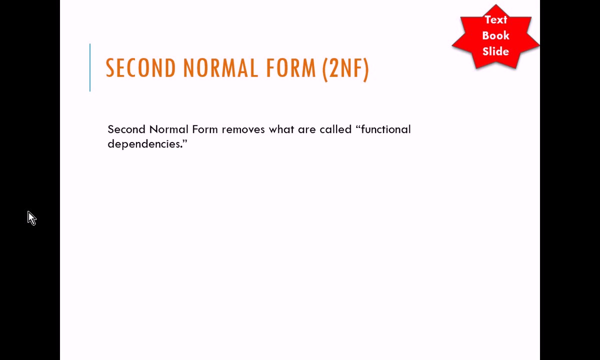 is referencing the album table. So now in our album table we don't have a list of tracks. Instead, they're all in this track table, which references back to the other table. So this would first normal form. Second: normal form removes what we call functional dependencies, which are: 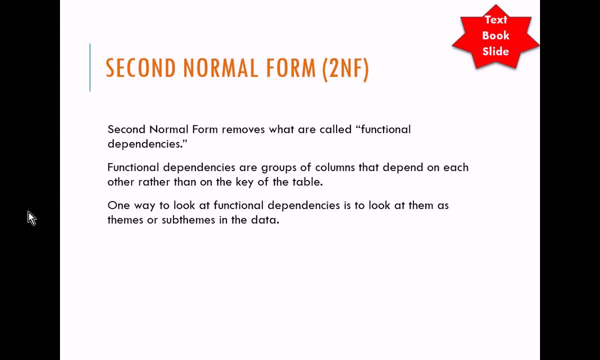 groups of columns that depend on each other rather than on the key of the table. So one way to look at this is themes or sub themes of the data, which we did before when we do our analysis. So, for example, on the album table tracks represent a separate theme or a functional 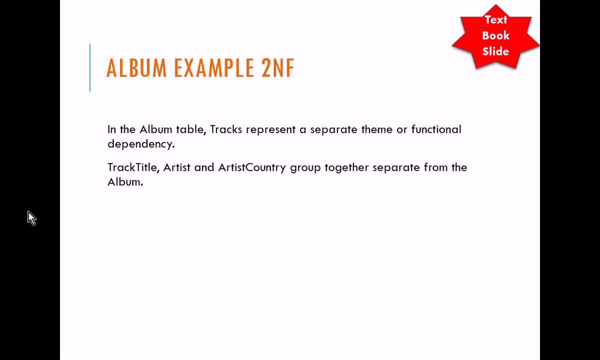 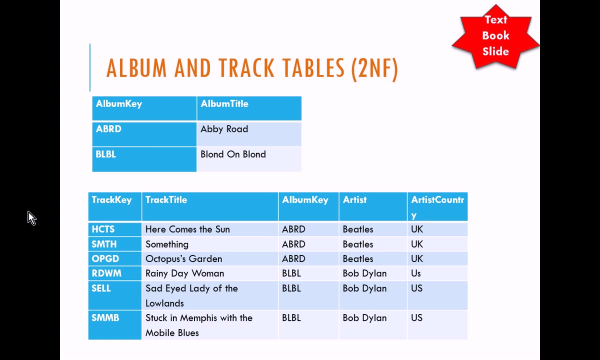 dependency: Track title, artist, artist, country. they can group together separate from the album table, So we can add a key to the album and track tables. So here we have our album table, There's our track table And if you look, we have our album artist now in that track table. 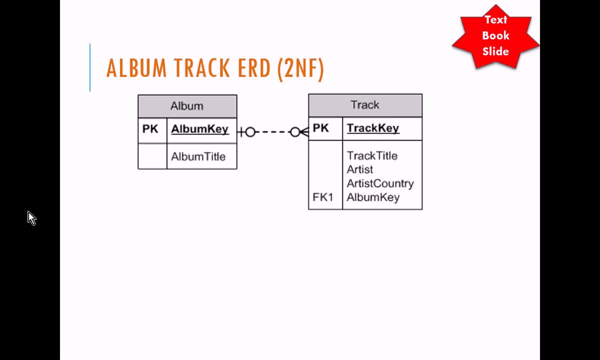 So we move the album artist over to the track table. So now we have an album which has a relationship to track. Okay, So we are in second normal form, So we're going to move the album to normal form. But to move to third normal form we have to move functional dependencies, or I'm 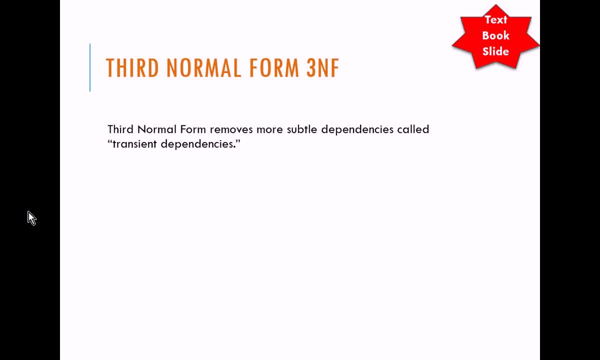 sorry, transient dependencies which are a little bit more subtle than our functional dependencies. So a transient dependency is where a field depends more on another column for its meaning than the table key. So, for example, our artist, an artist country, does not depend on the track. 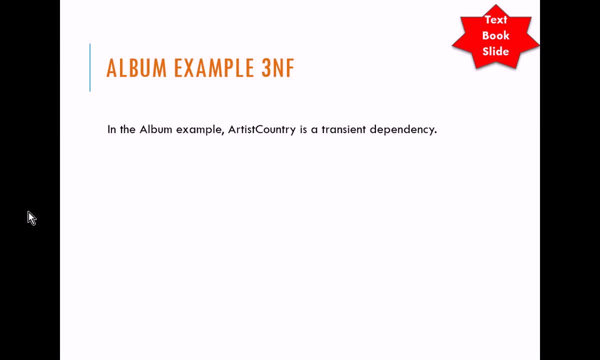 of the album that was written. It depends on the artist itself. So there's a hidden entity in our track table And we have to move the album to the track table. So we have to move the album to the track table And we have to move that entity into its own table. So we're going to create an 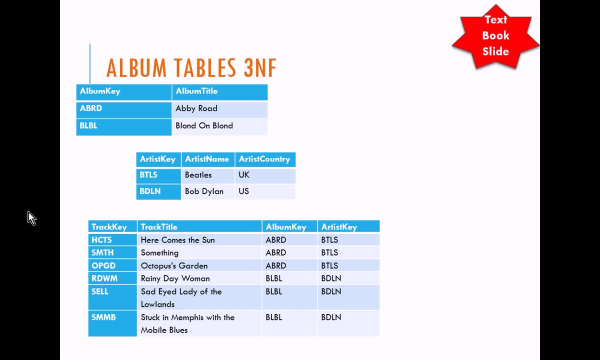 album artist table. So now we have an artist table, which is right there in the middle, And we reference that from the tracks. So at the bottom we've got our tracks. The tracks reference both the album and the artist that wrote the album. So that's an example And if we were going to look, 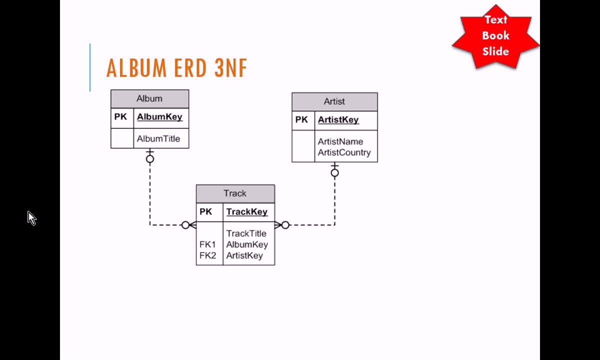 at that in an ERD or an entity relationship diagram. this is what it would look like. So our album can have zero or many tracks. Our track can have zero or many tracks, So we have an entity that has zero or one album. Likewise, our artist can be on zero or many tracks And our track has. 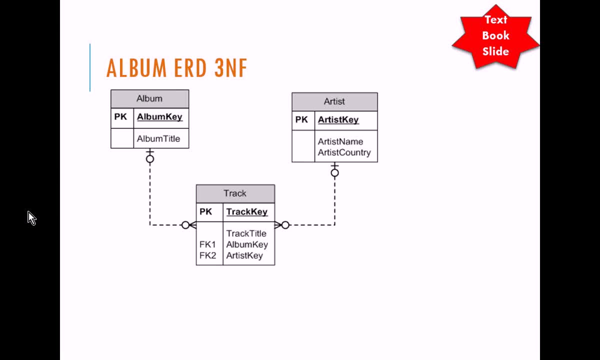 zero or one artist Notice here that we don't have any many-to-many relationships anymore. So this kind of worked out that problem of the many-to-many relationships And now we have these references to other tables. I'm going to talk more in the next video about how to create. 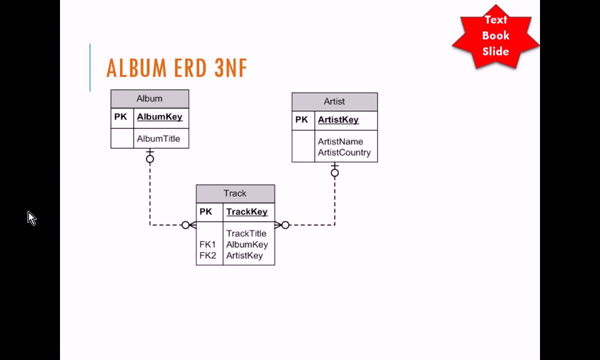 these foreign keys and make sure that the foreign keys are correct. But as a shorthand, I can tell you right now that if you're curious as to where your foreign key goes, this is a good way to figure it out. So here's a good example in this image here. Take a look at the relationships in 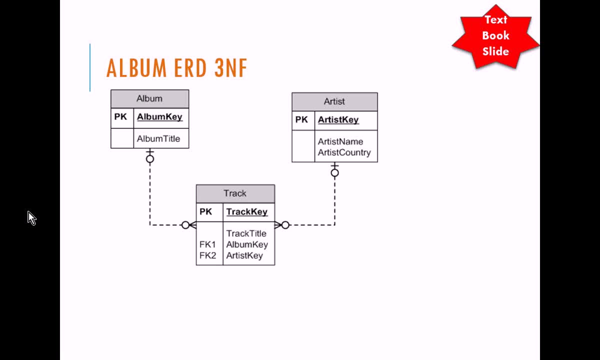 Crow's Foot, Where you see the many side of the relationship in Crow's Foot is where the foreign key has to go. So anytime you have a many-to-one or one-to-many relationship between two tables, take the primary key that's on the single side. So look on the right side, You've got artist. 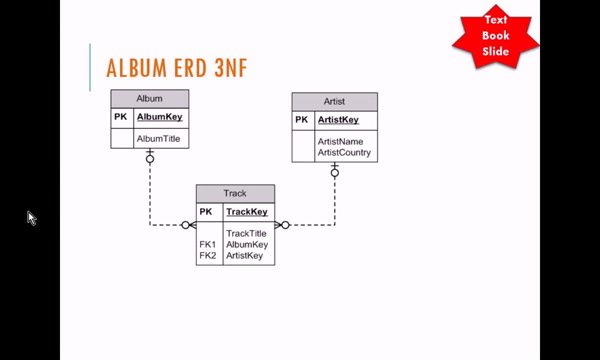 which is the single side. That's the one with the two-one relationship, That primary key, and we put it in the table on the many side. Likewise we have the one relationship side of the album and track relationship. The singular side is on the. 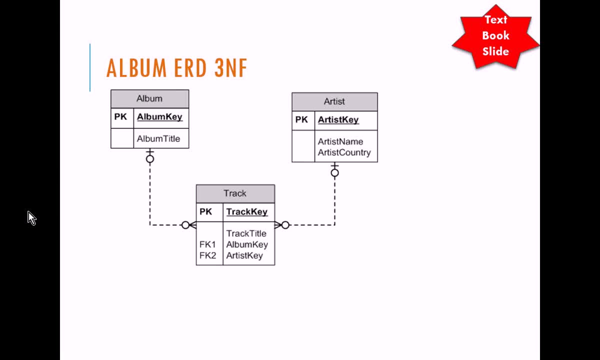 album side. So we take the primary key from album and we put that on the many side, which is the track side. So when you start doing your physical design to make sure you've got your foreign keys correct, anytime you see a one-to-many relationship, whether it's zero-to-many or one-to-many or zero-to-one. 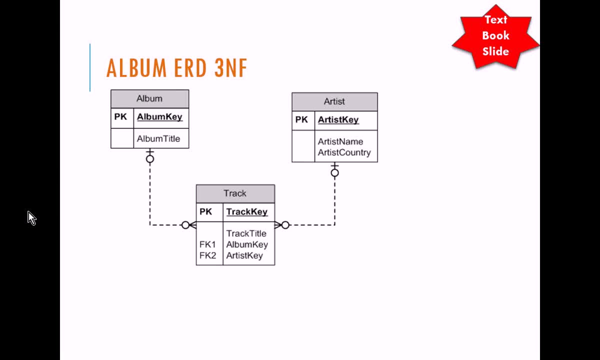 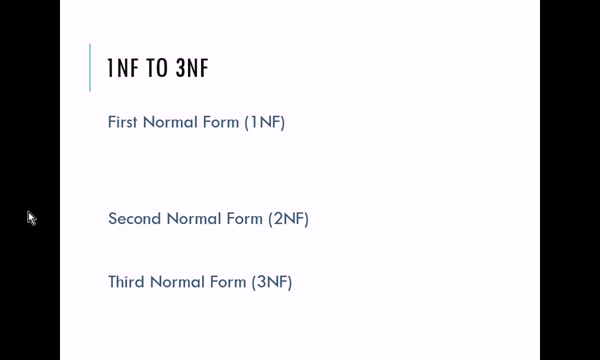 relationship, whichever side has the one, you're going to take that primary key and copy it as a foreign key in the many side And if you make sure you do that, then all of your foreign keys are going to be correct and everything's going to work. So that's third normal form. So I also have 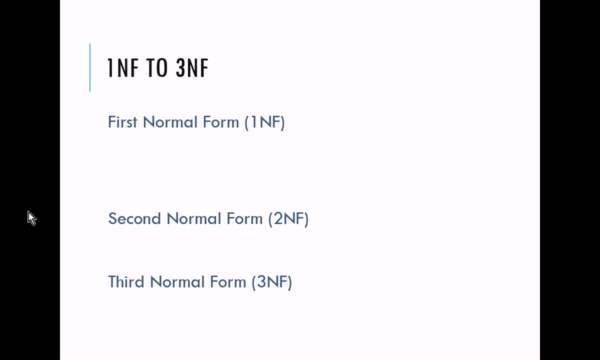 an additional couple slides, because I like to show this a little bit different. The slides I was showing you before are from a textbook. I'm going to give you kind of my more informal way. think about normalization. so it's a little bit different, But again we have these three normal. 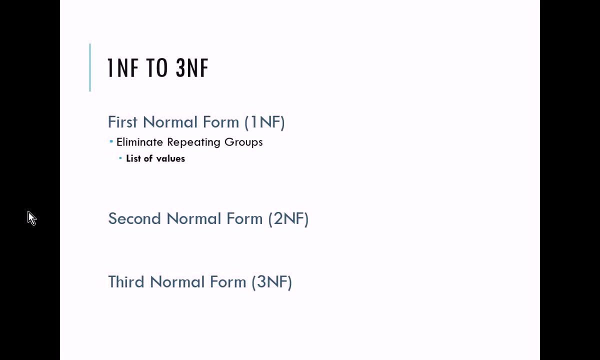 forms. You have first normal form, which is eliminating repeating groups or arrays. So I like to think of that as any list of values, enumerated fields like field one, field two, field three. Anytime we're listing something horizontally in a record, so when you're looking at the table, 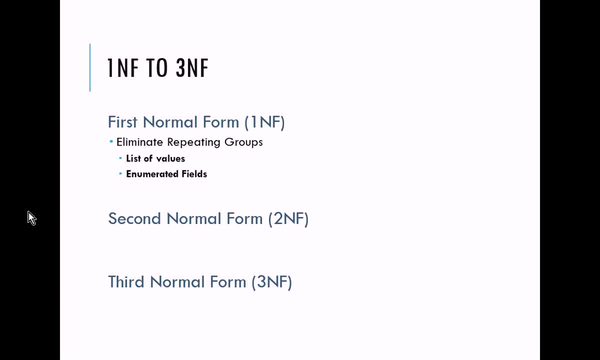 itself. if you see something repeating horizontally or across the screen, then you need to do something like that. So I'm going to get that to. first, normal form. Each field should always be a single data type. Second, normal form is where we remove the functional dependencies, So any groups of columns. 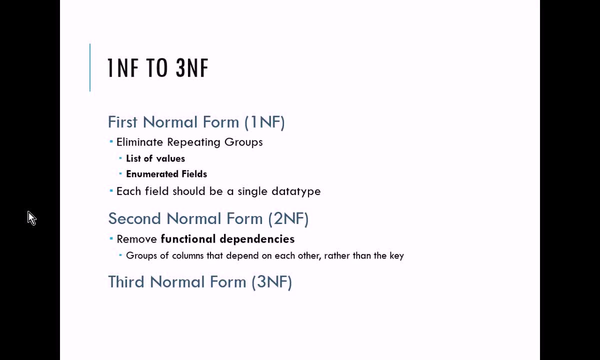 that depend on each other rather than the key. we're going to eliminate those. And then, finally, third, normal form is removing those transient dependencies where a field depends more on another column rather than the primary key itself, which is a little more difficult to see. that And 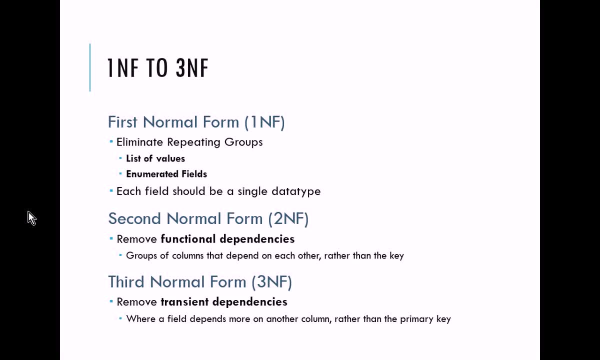 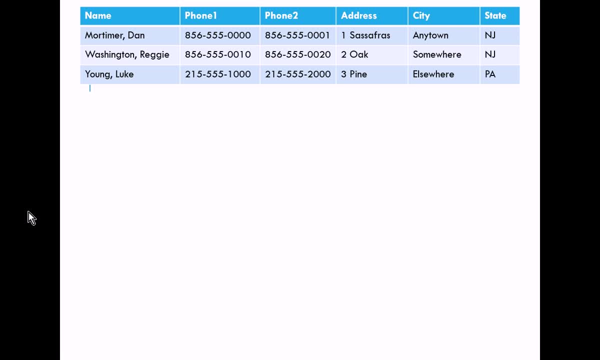 it's also not as critical sometimes to get all of those, but I'll show you why in just a few minutes. So take this example. Here we've got a list of students and you've got their name. on the left-hand side They have a phone one, a phone two, an address, city and state. Now you'll notice that we have 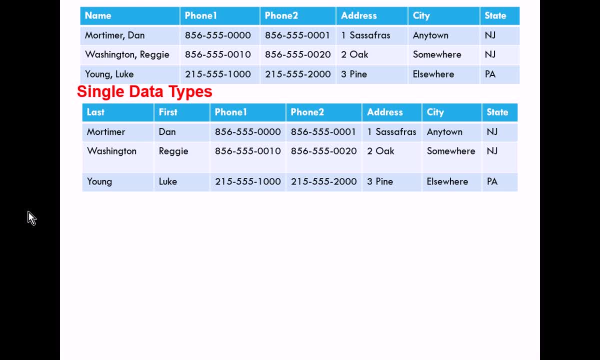 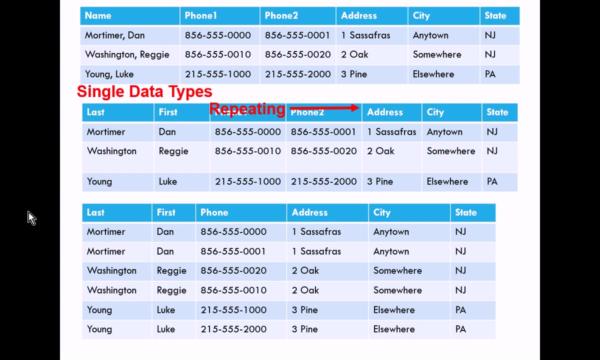 some problems here. The big problem here is: look at the phone number. So we have a repeating column in the horizontal direction. So when I look at a record going left to right I see the same data type repeating, in this case the phone number. So I have to eliminate that repeating value. So how do 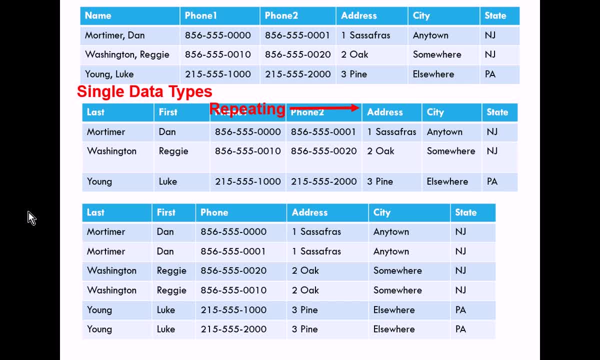 I do that. Well, one way to do that is to consolidate into one column. We'll call it phone. And now. now here's the problem is, now that I've consolidated into one column- and I have at this point- I now have first normal form. it's now repeating in the vertical direction. So now I 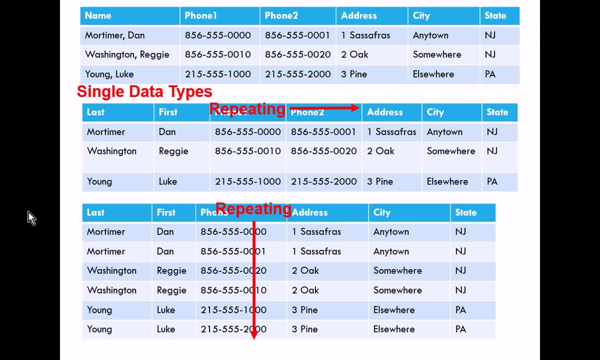 see repeating records in this direction. It's no longer, there's no longer a dependency there. So now I have to. I have a functional dependency problem that I have to eliminate because I'm duplicating records. So I have to eliminate that. So I have to eliminate that. So I have to eliminate. 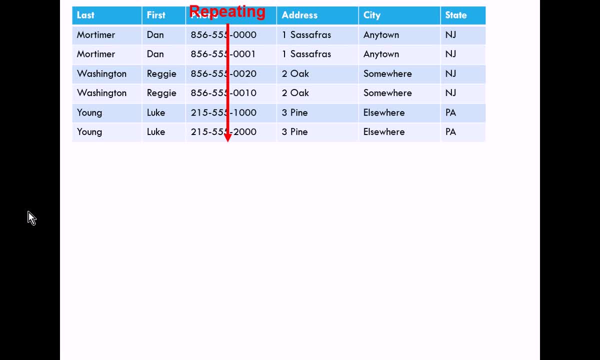 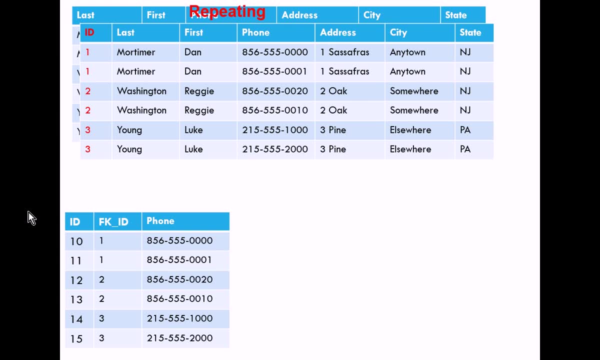 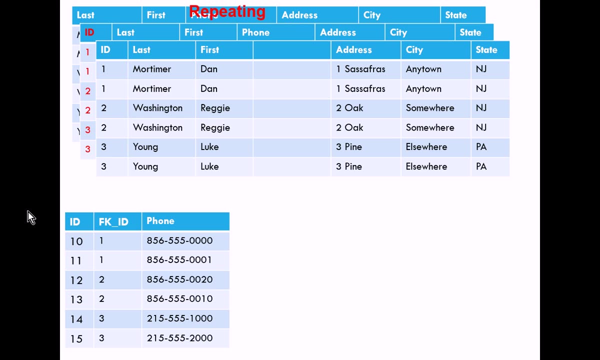 in order to support these multiple phone numbers. So to fix this and get the second normal form, I'm going to take the phone numbers and move them to a separate table. So now I've moved those to a new table. That's how I I get those phone numbers out of that table And now I can consolidate down. 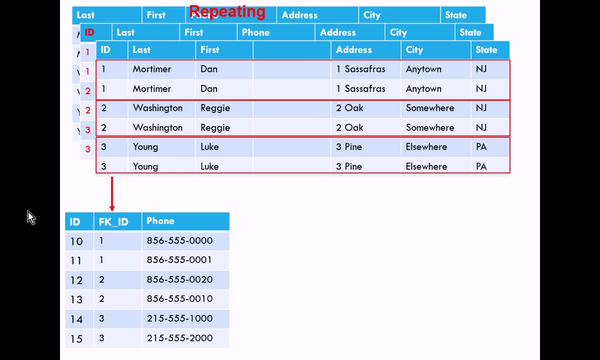 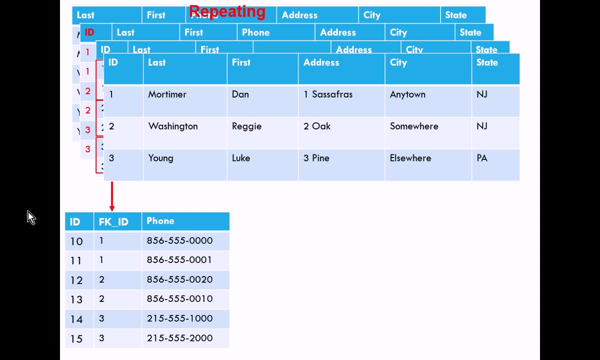 So my phone numbers are out now. So now I can go back to my single records. So let's take a look at that. So now I have my one record, um, and they are referenced from the phone table. So in my phone table I have phone numbers for all of my students And if they have more than one phone, 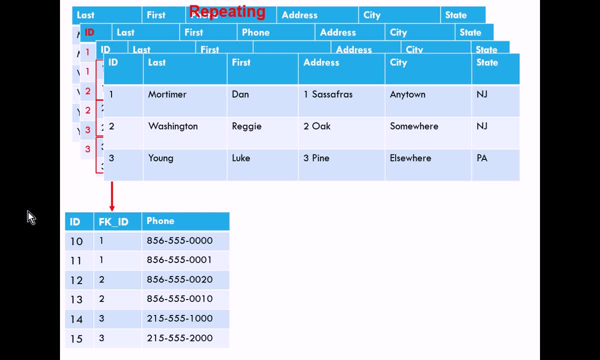 number. that's okay. I can have them multiple times in that table because there is no dependency problem, no functional dependency problem there. Every single phone number in that table at the bottom is dependent on its primary key on the, uh, the ID that you see on the left. So now we've. 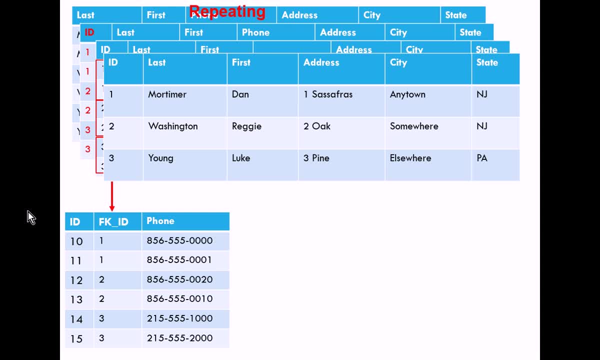 eliminated both the repeating sets on the horizontal direction and the repeating sets that happened in the vertical direction. Um, and a lot of times, when you're going from, uh, a non-normalized to first normal form, uh, when you go, you'll be creating a problem that. 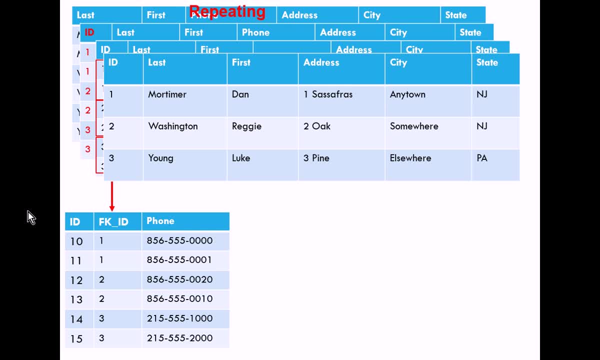 then has to get fixed with second normal form, which we've just we've just done here. So the next step: now we have a problem. So we are in second normal form at this point. but take a look at that table and think about: is there anything in that table? uh, that is not dependent on the 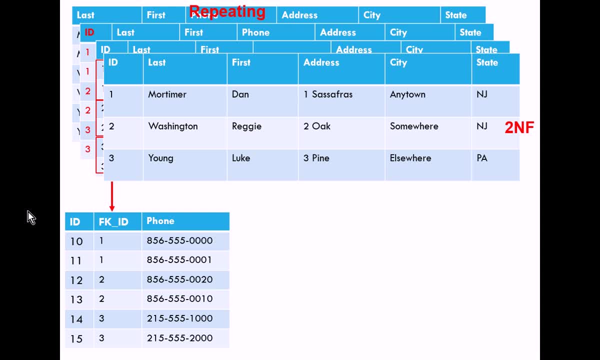 person itself. So- and the answer is yes, there is. So, for example, the address, city and state. that is a hidden entity, right? So so that's an entity in and of itself. the address, city and state. It's not wholly dependent on the uh, on the ID You could have multiples people living at. 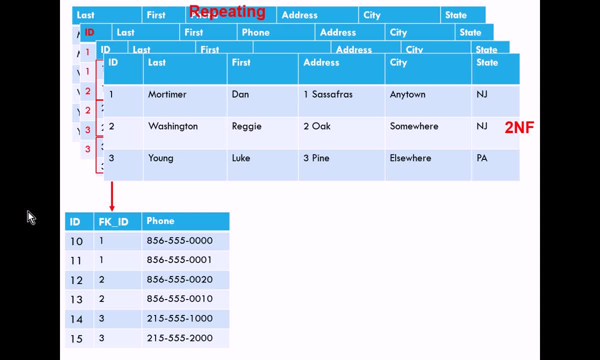 the same address. What if you had two students that were brother and sister? they would have the same address, right If they were, if they lived at the same place. So there's a dependency, there's a there's. there's a transient dependency there that we have to fix. So how do we do that? 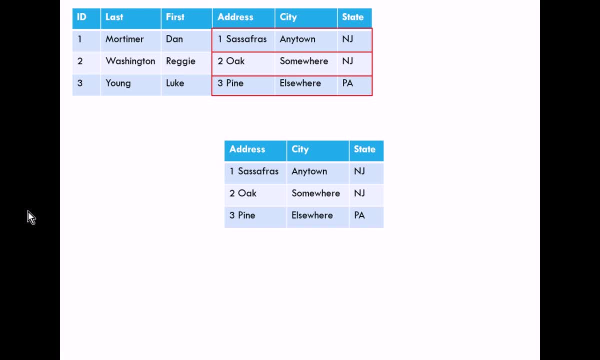 We take the address and we move it to a new table. So and you're probably getting the idea here that normalization involves creating lots of new tables- and there's definitely some truth to that- So you will find yourself creating some new tables when you're doing normalization, for sure. So we've moved these to a new table, So now they're gone. 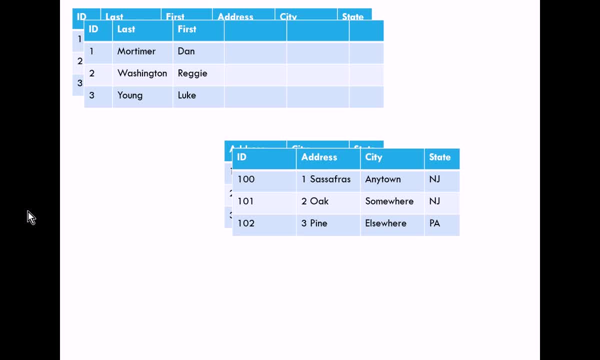 Uh and instead we are going to reference uh, our, um, our address. Okay, So now we add the address to our student table and it references the address table itself because we added an ID number one. Dan Mortimer, uh, has a uh address ID of 100, which references one sassafras in any. 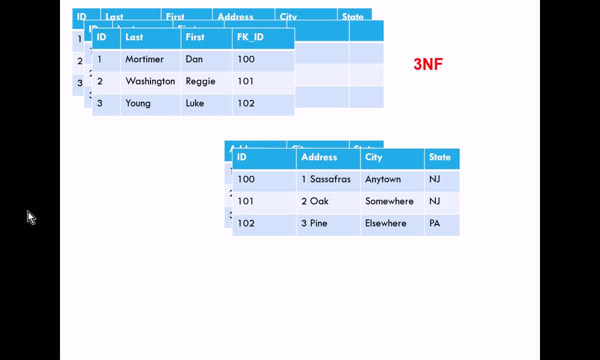 town in New Jersey. Now that's third normal form And in theory we could keep doing more third normal form normalization here. If you look at the address table now, there's an additional dependency here. What about the state? I've got repeating values now for the state. The state is. 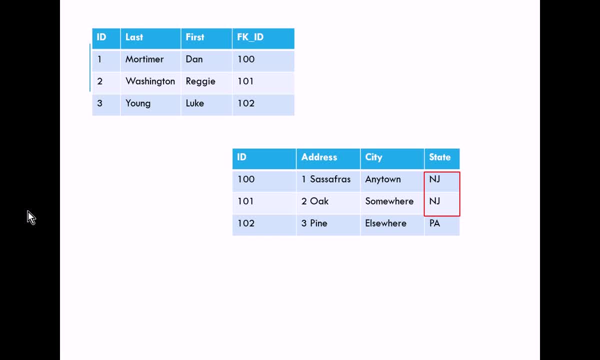 not dependent on the city right. So cause there could be lots of cities that have the same state, So we can keep doing more. third, normal form normalization. here If you look at the address table state, So in theory I could move that to a new table right. So here I've moved that to a new. 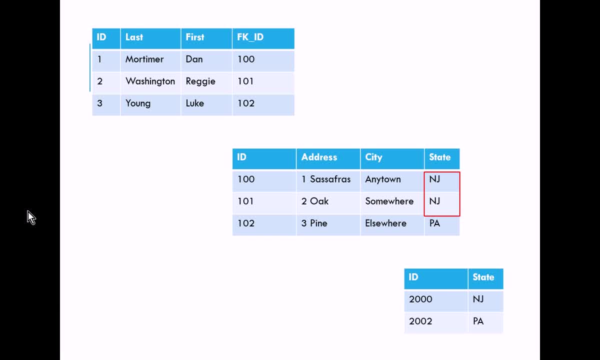 table And technically that is normalization. doing that I've, I've further normalized this database. It's still in third normal form, Um, but I could keep going, I could keep pulling things out that look like transient dependencies, but you know, and for example, the city, I mean. 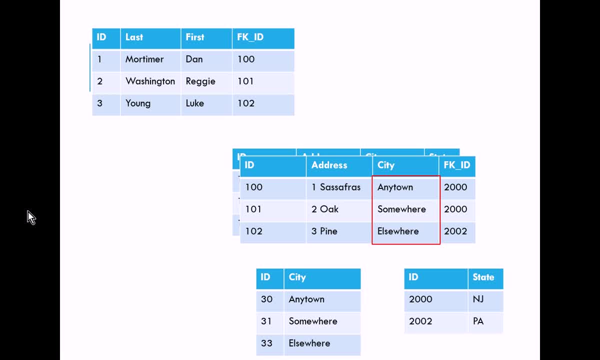 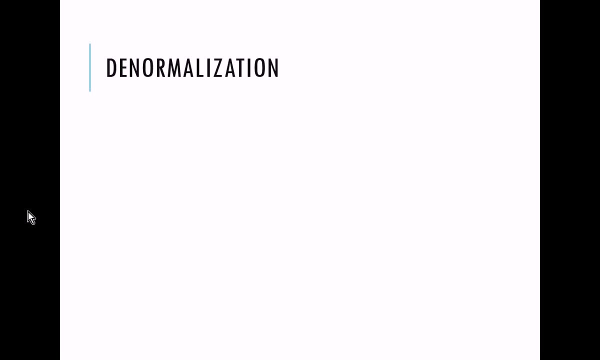 there could be students to live in the same city, So we could have an ID for the city and then and then reference the city ID. If you keep doing this, you can end up with hundreds and hundreds of tables with all of these foreign key relationships. 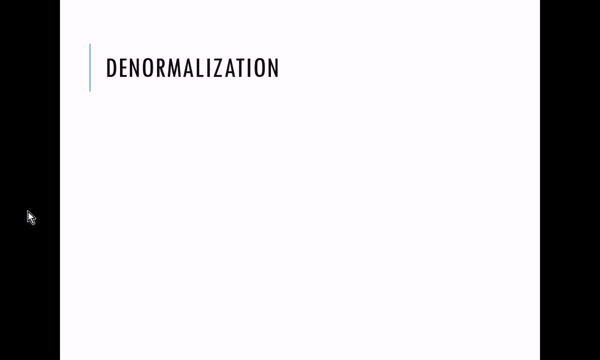 The more you normalize a database, the more resources and time it takes to get information out of our database and to insert information to our database. It gets a little bit more time consuming to do all that stuff. So at some point we have to say: you know what we've normalized. 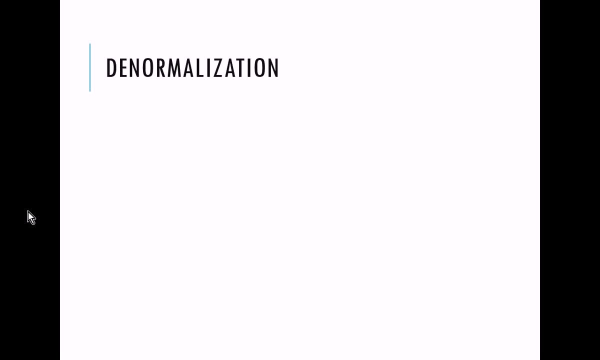 too much, So you may denormalize to get back your performance of your database. So, even though you're going to have, say, a lot of data- you're going to have a lot of data- you're going to have a new Jersey in your database many, many times. Um, maybe that's a field that you don't want to. 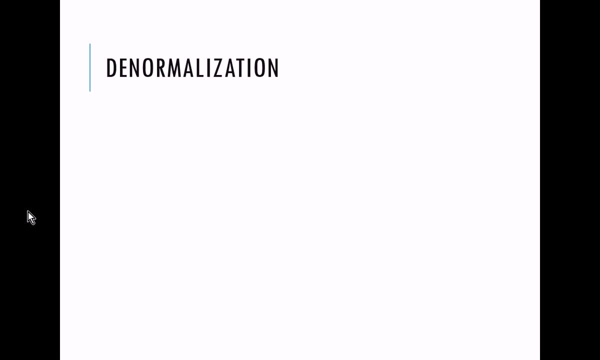 have in a separate table just because it's one more join you're going to have to do And you're going to have other things in place that are going to prevent any kind of inconsistency there. Uh, so that's what denormalization is And it's going to, and we're usually going to do this for. 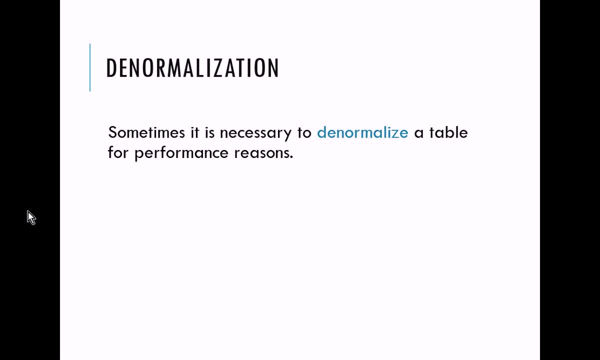 performance reasons and for simplicity, because sometimes it's just too many tables. It's just going to get ridiculous. I've worked with databases that have tons and tons of tables and it's very confusing to work with them when they have a lot of data. So I've worked with 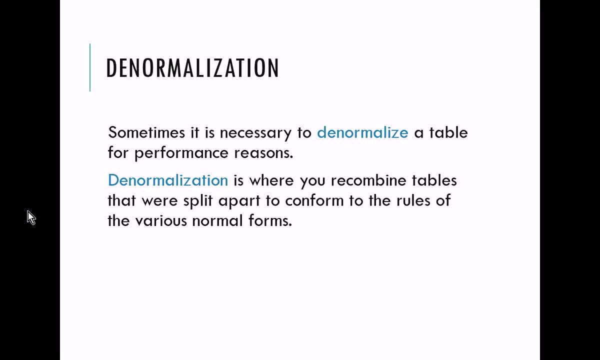 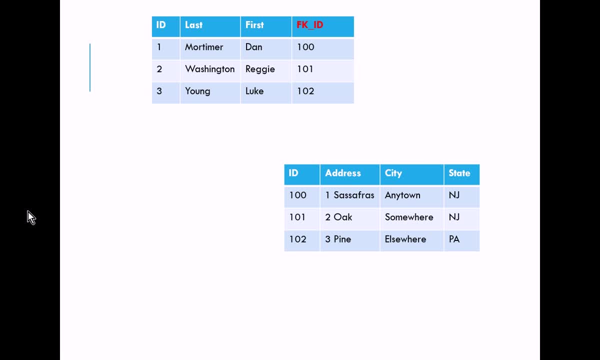 a lot of tables like that. So we recombine tables that were previously split from our normalization uh in order to make the database uh perform a little bit better. So in this example, we can always move back uh our address, our city and our state back into that address. 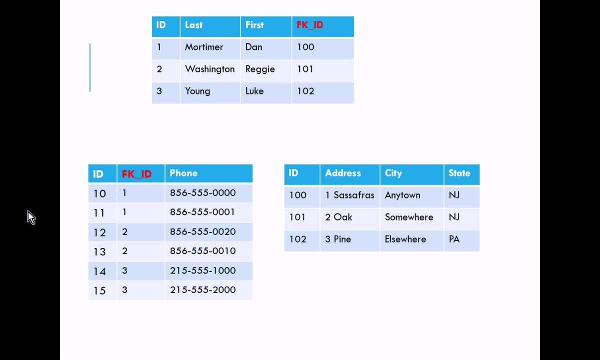 table, because it simply isn't necessary to have it in a different table. All right, So we also. so now this is our final design. This would be our normalized design, because we denormalized a little bit, but we're still mostly in third normal form. We're going to connect. 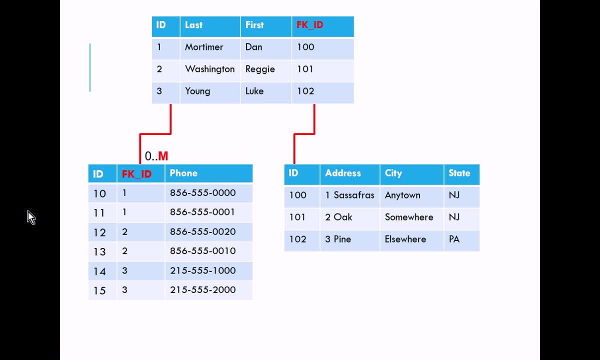 uh, these tables and put our relationships back in. So our student can have zero or many phone numbers, Our phone numbers can have one and only one student, right? Um? our student can have one and only one address, and an address can appear on one or many student records. Now, once again, 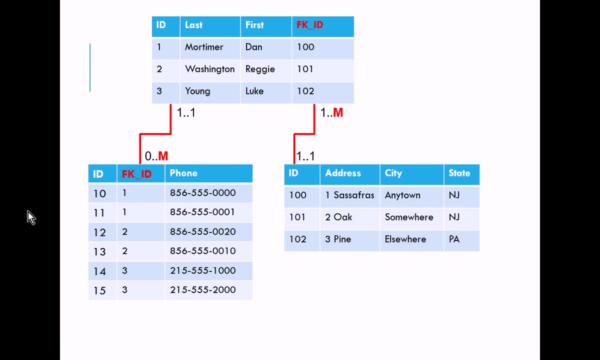 I want you to notice that the? uh, look at the the many side of these relationships, right? So take a look at the Ms on here and look at the foreign keys. You'll notice that foreign keys are referenced on the M side. Okay, So if you look at the phone, the phone. 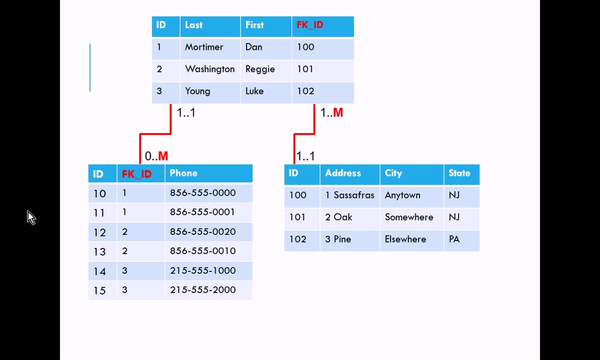 number. for example, there's an M on the phone number side, the many side of that relationship, and the crow's foot. that's the symbol that looks like the crow's foot, the three little lines the many side. on that side of the relationship I have the foreign key. I'm referencing the primary. 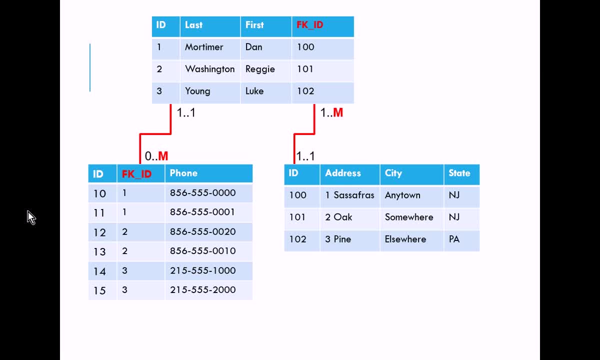 key from the student table which I have that line pointing to that key to make it more clear here what's happening. Likewise, if you look at the M on the student table, that foreign key references the primary key on the address table on the. 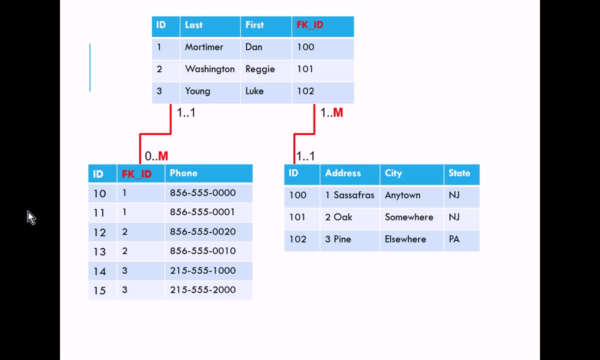 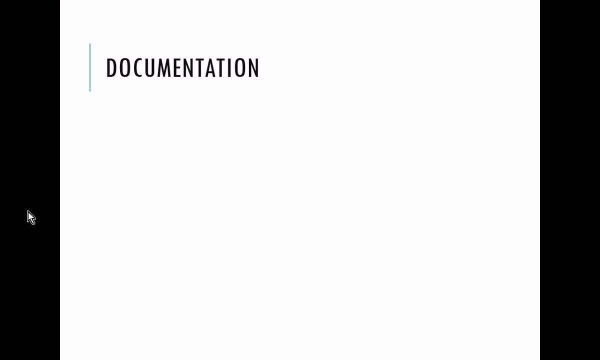 one side. Okay, So that's a nice shorthand for where to make sure you're putting those foreign keys, making sure that they're in the right place. Finally, documentation: as always, documentation is important in uh database design. You should keep every version. 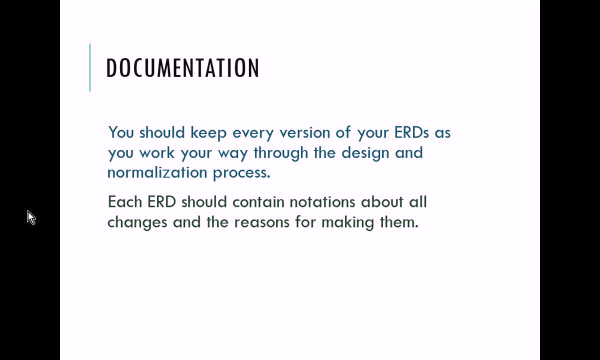 of your ERDs, as I explained in the last video. uh, cause you're going to use them later on, especially at this point, because now, once we've normalized our database, we're going to make sure we have our database. We've added our foreign keys, which I just talked about. 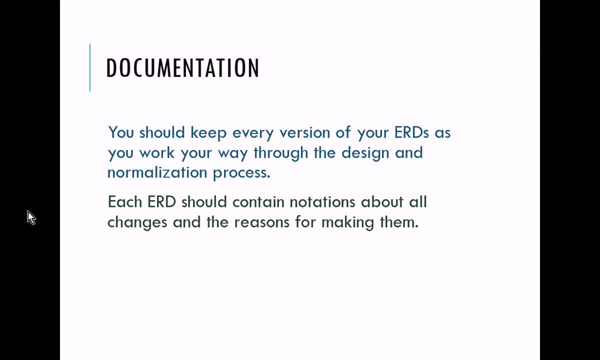 So we're going to make sure we have our foreign keys and um you know they're correct for the types of relationships that we've identified. We have all of our attribute names in there. We know the data types that we're going to use. We pretty much have everything we now need to build. 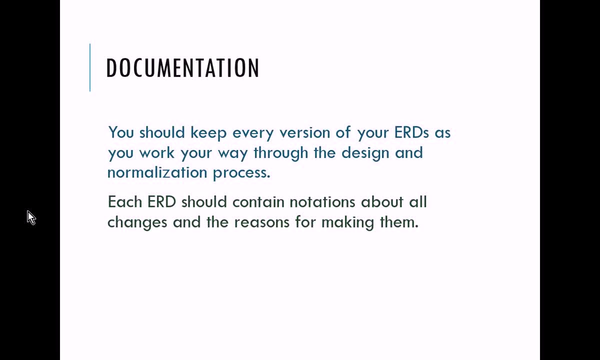 our database, which is what we talk about in the next video. We're going to talk about how to actually take this design that we've done and use that to create our database. So, again, documentation is important and we're going to use.